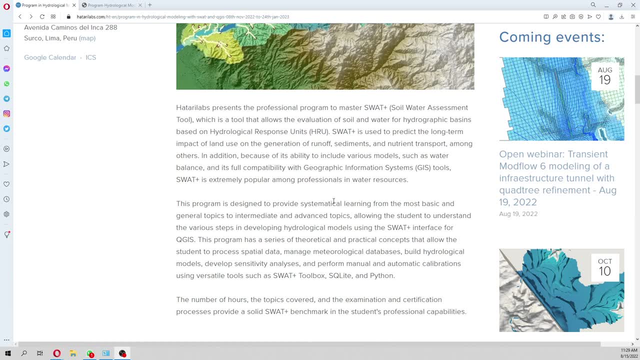 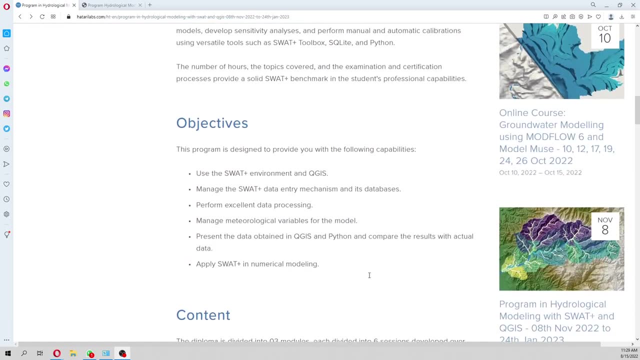 sensitivity analysis and perform manual and automatic calibrations with the SWAT plus toolbox and SQLite. Thank you, and Python. The objectives are to manage the SWAT plus environment, manage the data entry mechanism, perform data processing, manage the meteorological variables and present the data. 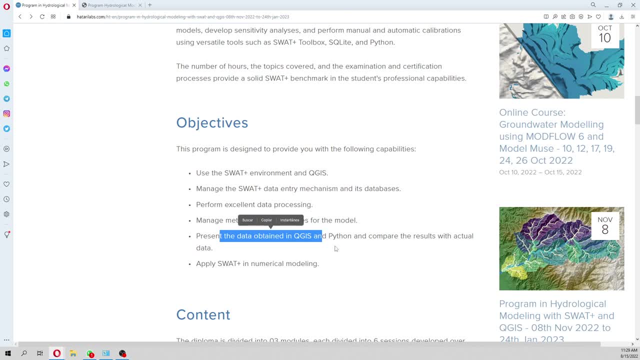 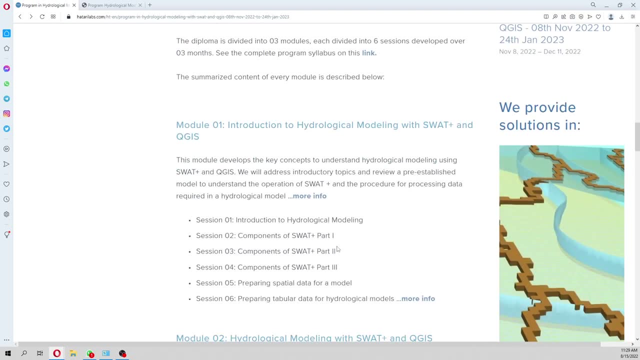 obtained- I mean the output data in QAAS and Python- And the program is divided into three courses. The first one is a course for that develops the component of the SWAT Plus and prepares special data and prepare tabulate data for the hydrological models. 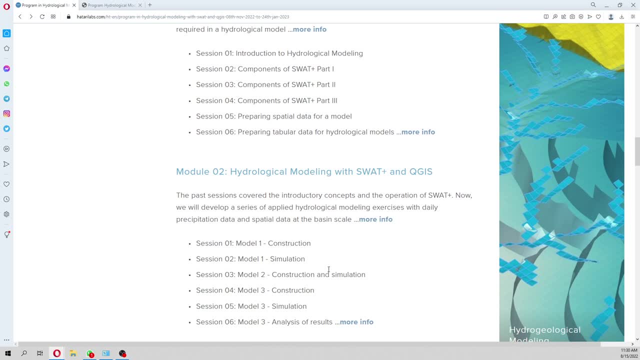 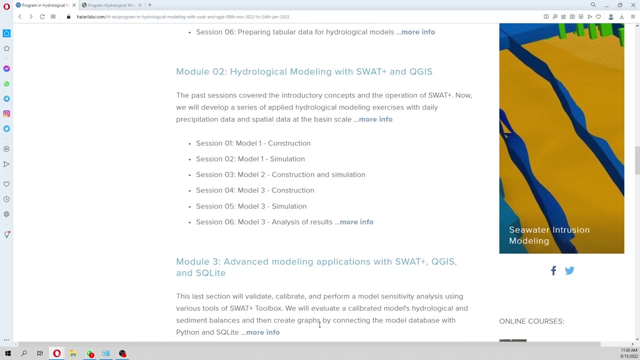 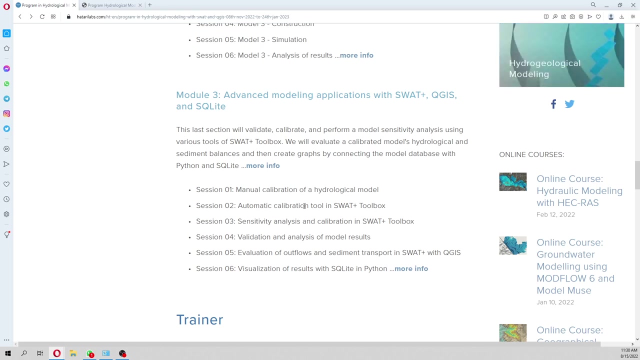 The second module develops three cases. okay, So it has model one, model two and model three, While The third module develops more intermediate and advanced topics as manual calibration, automatic calibration, sensibility analysis, validation, analysis of model results and visualization of data. 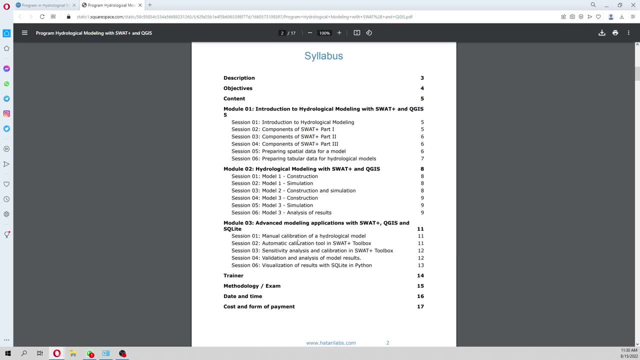 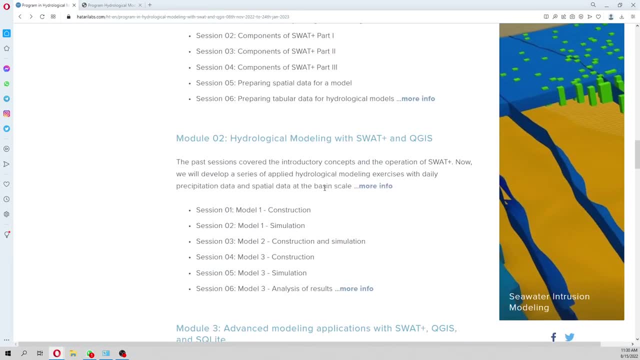 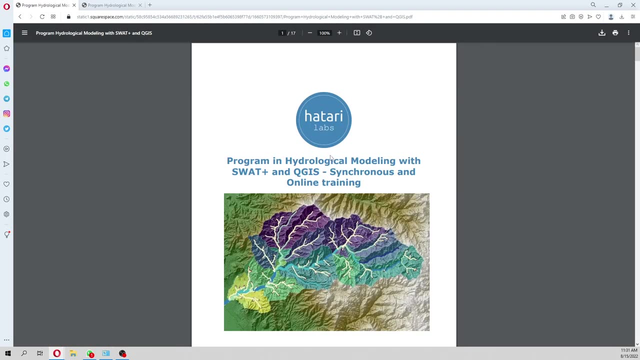 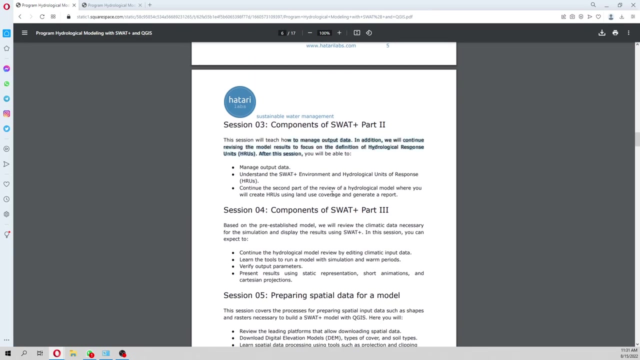 The whole, I mean the whole program, together with the content of each class, is developed here in the. you can find it here on this link, where you can find the for each class, which will be the what we are going to do in each class and together with some well. 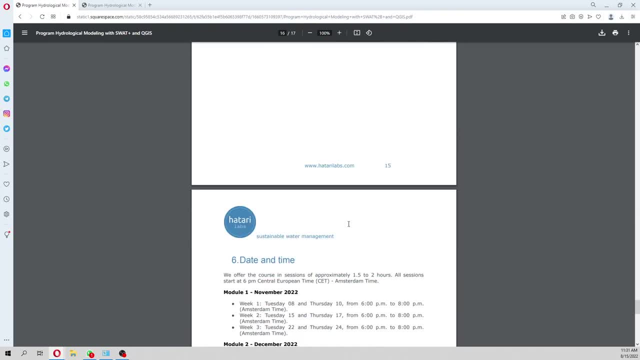 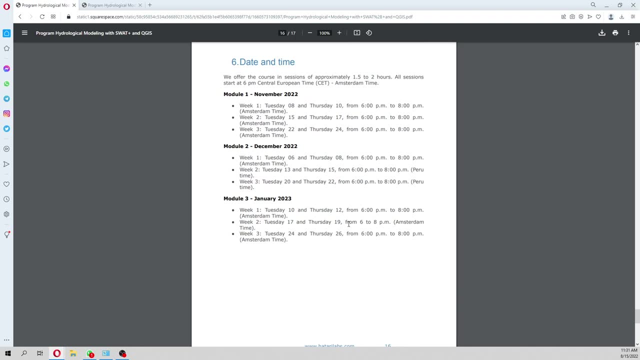 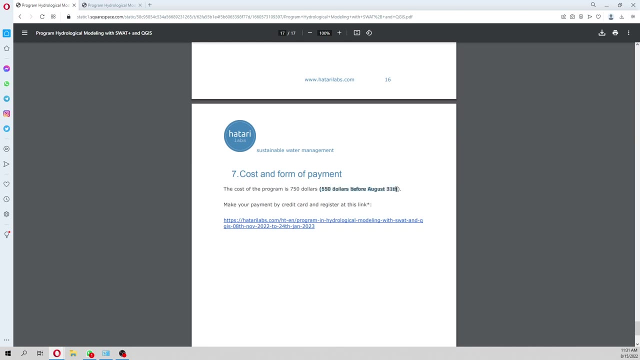 for the three modules. ok, with some other relevant data. the dates that would. this is going to the dates of the of the classes and as well the course. Please take advantage of the discounts if you pay with anticipation, and we hope to. 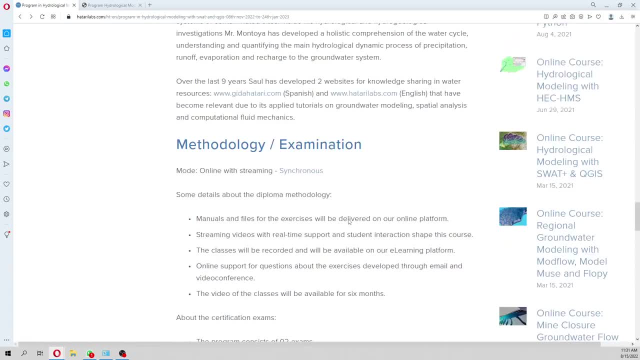 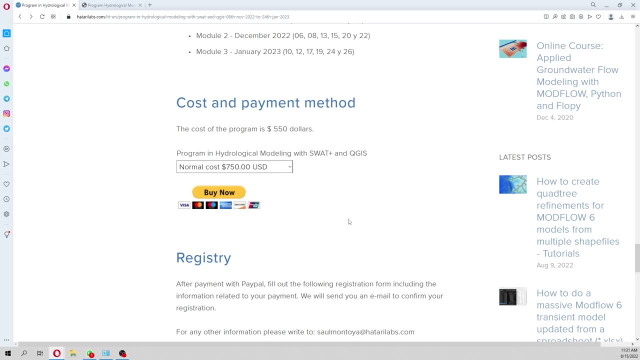 see you there in the course, because this is a very applied course and is kind of the unique course in its in the environment of online training. It is a very good course, SWAT+. Okay, my name is Raul Montoya. Please have a great day and hope to see you in the course. Bye-bye, Bye.